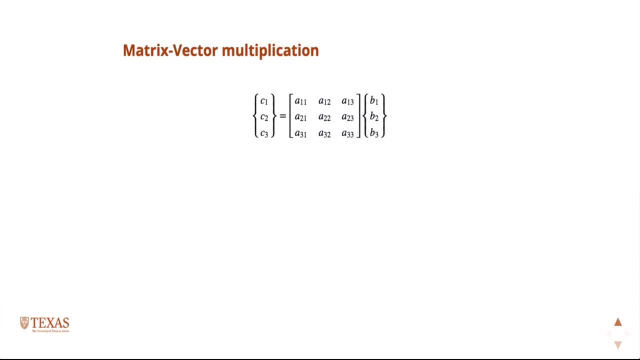 So those of you that know some of this, you might be bored, but understand we're working up to eigenvalue problems. So if I have, if I have, a vector C, we normally write this in vector notation: vector C, a matrix A and a vector B. 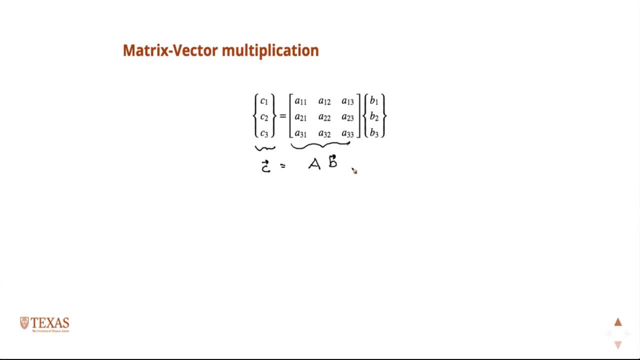 I want to do a matrix vector dot product, essentially The way I compute the components of C, and I like to remember it like this. I like to use words, I like to just say it in words. So so, C1, the first component of C is the first row of A dot product B, right, 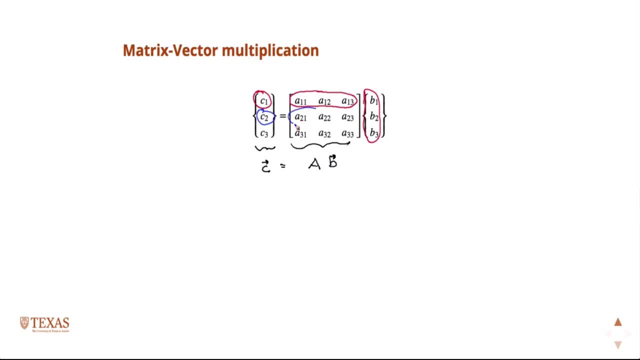 The second component of C is the second row of A, dot product B. You all know what a dot product is, And you know. finally, the third component of C is the first, the third row of A, dot product B, And so there's what it is written out for each component. 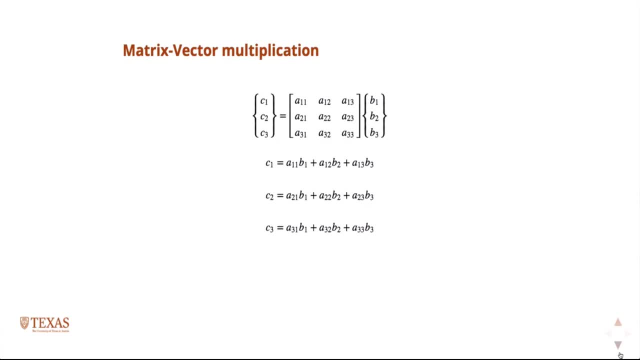 Everybody. okay, Matrix vector, dot product. So I figured you probably know that. So in words, the CI. right, so I be the ith component of the C vector. The CI is the dot product of the ith row of A with B. 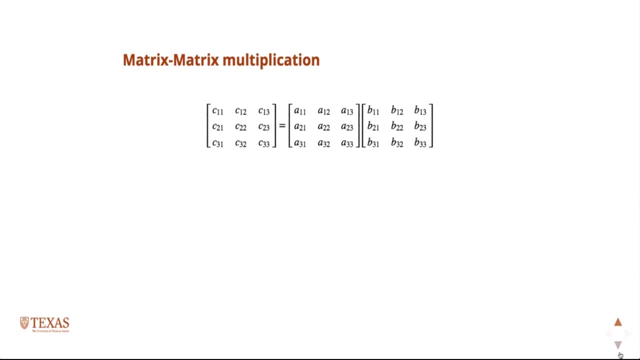 So you probably all know that. but what you may not know is you know how to do matrix, matrix multiplication. So in a matrix, matrix multiplication- again I like to use words. so the C11 component of C, right. so now we have three matrices, right? 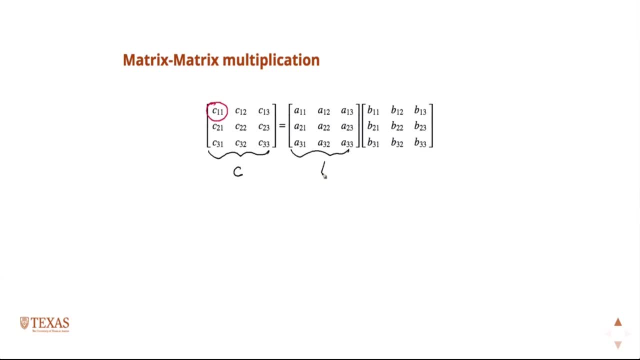 So this is a matrix C, a matrix A and a matrix B. So the C11 component is the first row of A dot product, The first column of B. The C12 is the first row of A second column of B. 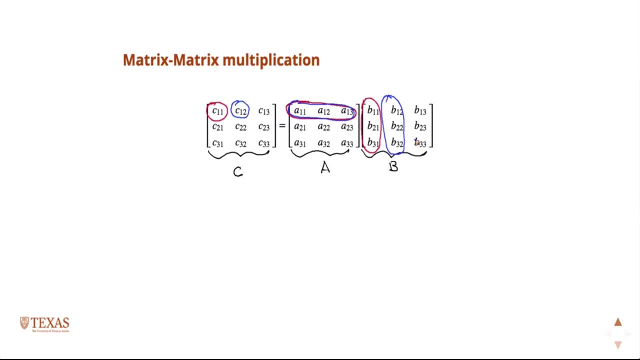 Right. C13 is the first row of A third column And these go on like that. So essentially you can look at the lowercase indices and tell you know this is associated with the row of A and the set. the first one is the row of A and the second one is the column of B right. 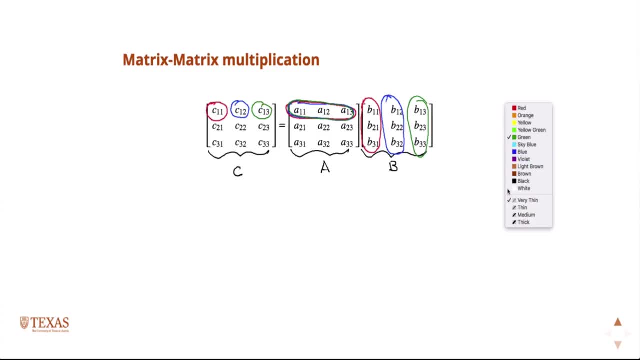 So, for example, to jump out of order, you know the C32 is going to be the third row of A with the second column of B. So, for example, to jump out of order, you know the C32 is going to be the third row of A with the second column of B. 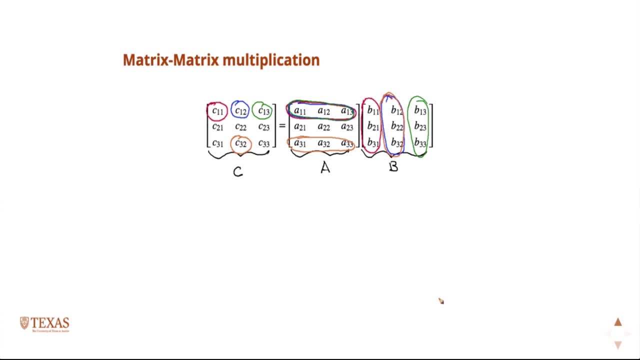 Dot product. So there's a couple examples written out: dot products. you know n-word, n-words. The IJ, where IJ is the component of the C matrix, the CIJ is the dot product of the ith row of A with the jth column of B. 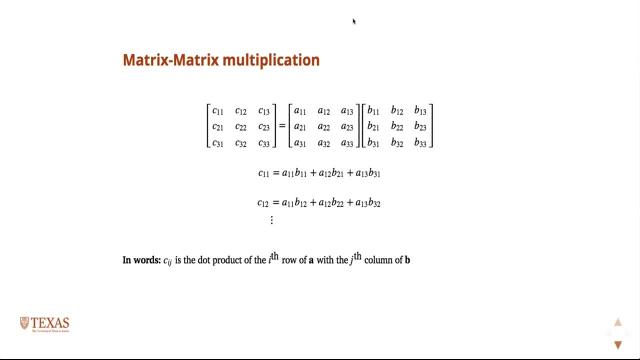 So well, I was going to work that out, but there's the answer. I meant to hold off on that, Yeah. so again, we take the first row here: 2, 1,. take the dot product with 1, 2, right. 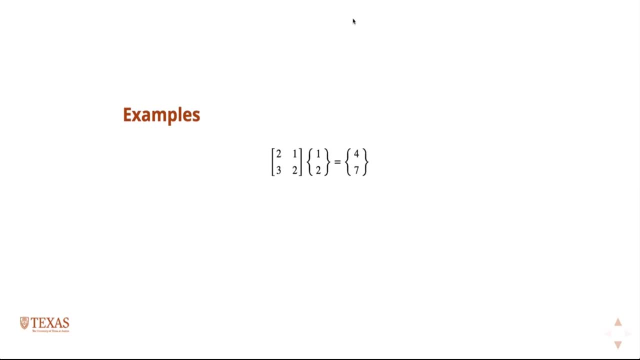 So that's going to be 2 times 1,, which is 2.. Plus 1 times 2,, which is 4.. Same thing, 3 times 1,, which is 3,, plus 2 times 2,, which is 4.. 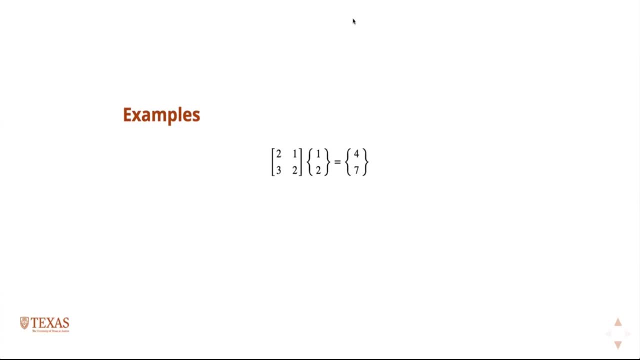 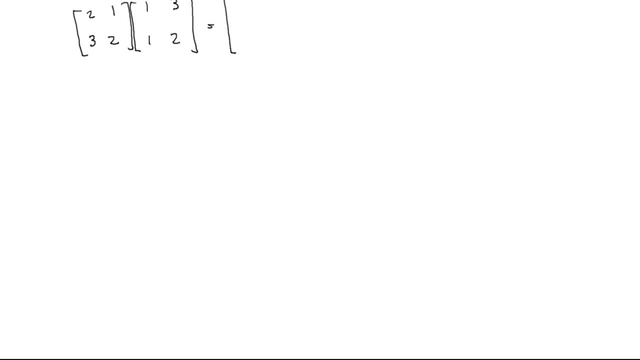 And I'm just going to write it out very explicitly here: go slow. So our result will also be a matrix. I've put the little dashed lines in it. We'll just separate the locations, the entries in the matrix, right. So we have for the first the 1, 1 entry. we have the first row of A right. 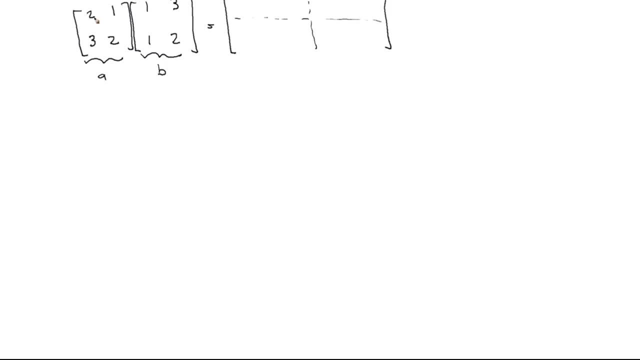 This is A, This is B. We have the first row of A with the first column of B, right. So that's 2 times 1 plus 1 times 1, right? And then for the 1, 2,, we have the first row of A times the second column of B. So 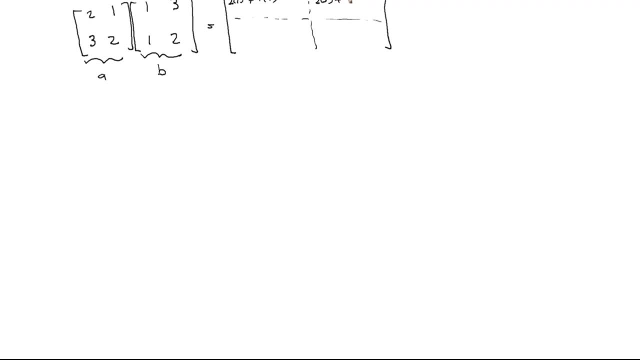 that's 2 times 3 plus 1 times 2, and then we continue right: 3, 1 plus 2, 1, 3, 3 plus 2, 2, and so then, if we just work out the math, you get 3, 8,. 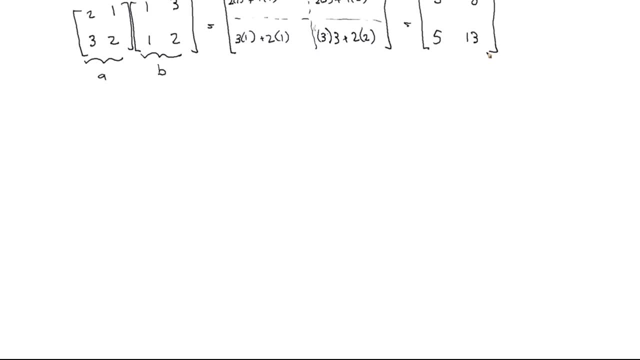 5, 13.. So that's the second example. So another useful thing in linear algebra is to take the determinant of a matrix. So who knows the formula for the determinant of a matrix? I don't, I don't, Okay. 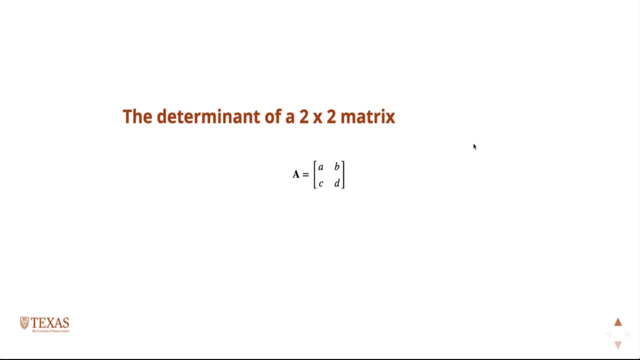 A D minus B C. A D minus B C, right, So you can memorize that formula if you want A D minus B C. I like to just kind of think of it graphically, right. 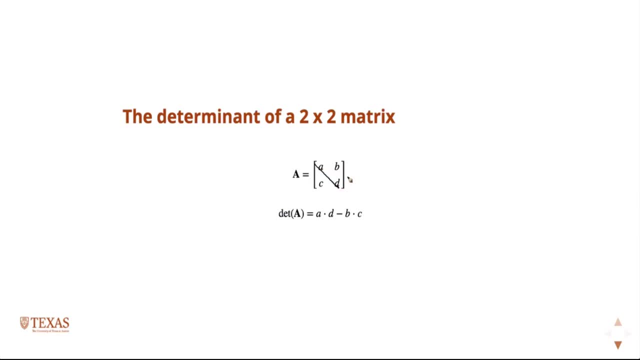 So I just make an X right. So it's A D minus B C. That's how I remember it. Just make an X. And the reason that helps me is because when you go to higher, bigger matrices you can sort of also. 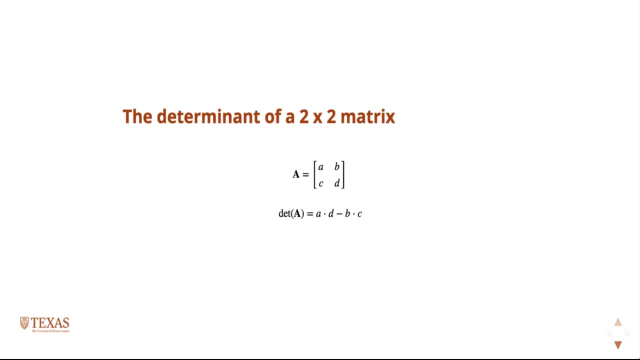 You can do it graphically. So for a 3 by 3 matrix, I mean you can memorize the formula if you want. There it is. I think it would be pretty hard for me to memorize that. But what I do is again just: I start with A, I start with A and then I cross out the. 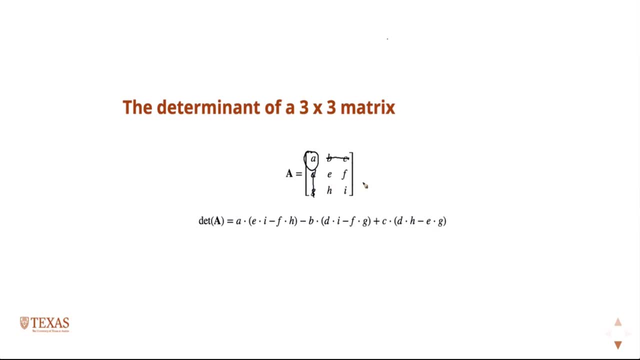 row and column, and then I take the determinant of what's left over and just use the X, EI minus FH. So that's that formula, okay. And then there is The thing you do have to remember is there's a minus sign. 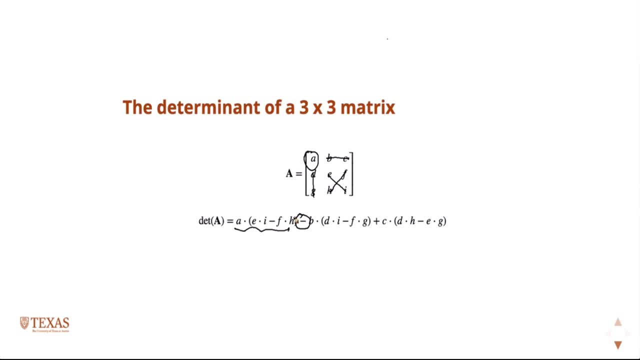 So they'll always alternate plus minus, plus minus, plus minus, and this generalizes to very large matrices. So then, for the second one, then I'm going to take B, I'm going to cross out the row and column and then take the determinant. 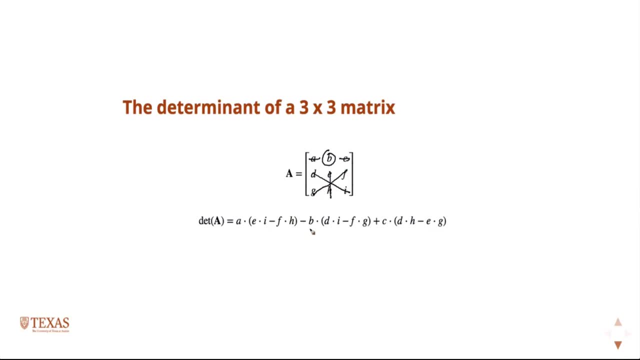 of what's left. So D times I minus F times H. That's what you have there For C. I'm going to cross out the row and column and take the determinant of what's left: D times H minus E times G. So then all you have to remember is just that it's going to 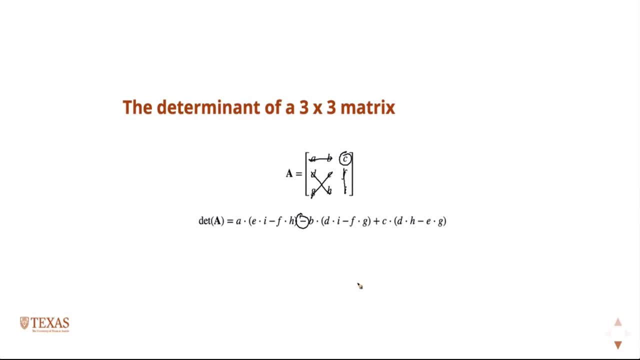 go plus minus, plus, minus, plus minus. And that generalizes, Because if I had a bigger matrix, like if I had a 4 by 4, I wouldn't recommend ever taking the determinant of anything bigger than a 3 by 3 by hand using a computer. 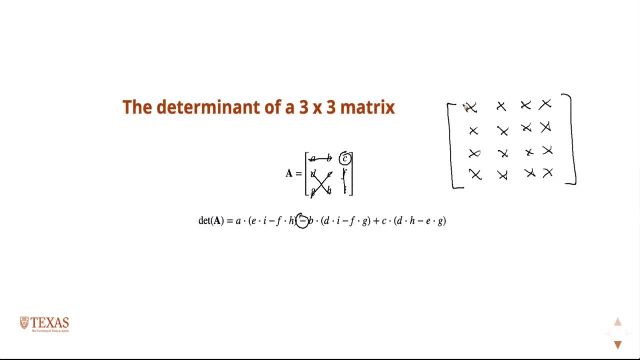 But you could do the same thing, right? So for a 4 by 4, you're going to take this guy times and cross the row and column out and then figure out what the determinant of that guy is, right? Well, the determinant of that guy. then you'd do this again, right? 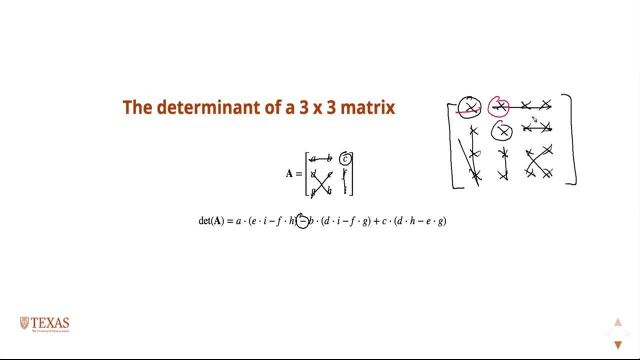 And then you'd go the same thing. right Now you'd have a minus sign, oops, and then compute the determinant of that 3 by 3.. Then you'd have a plus sign and compute the determinant of that 3 by 3, and this goes. 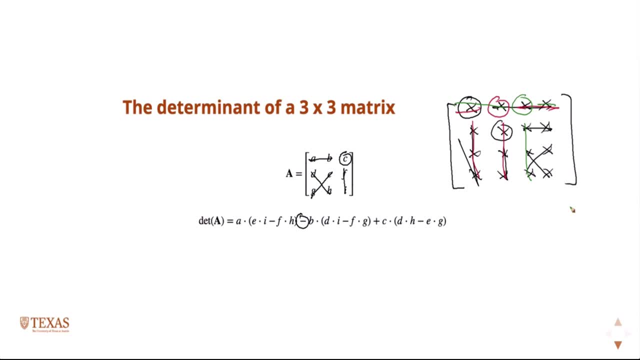 on and on. Again, I would never take the determinant of anything bigger than a 3 by 3 by hand using a computer. But if the computer doesn't actually implement this rule, like I showed, there's a better way to do it with a computer. 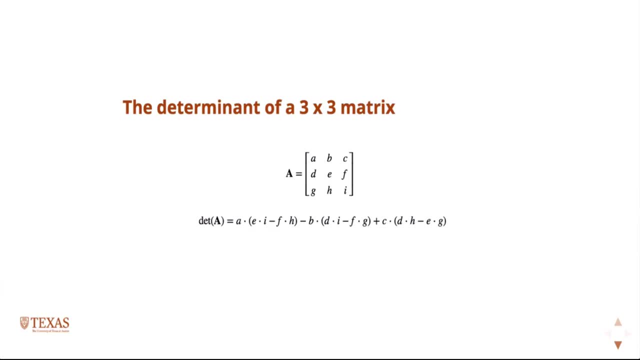 So one thing that's useful: what can we use determinants for? You know, when we solve linear systems of equations, we often solve a system of equations that has the form you know we're looking for. we're looking for the determinant of. 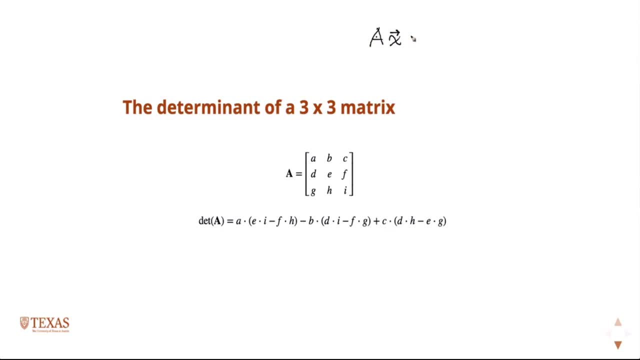 the solution: X for a matrix, A times a. vector X equal to a, vector B, AX equal to B. this is what we're. you know if you've taken- well, I guess only a couple of you took res 3 from me, but so far. but if you take res 3, I mean this is all we do. all class solve. 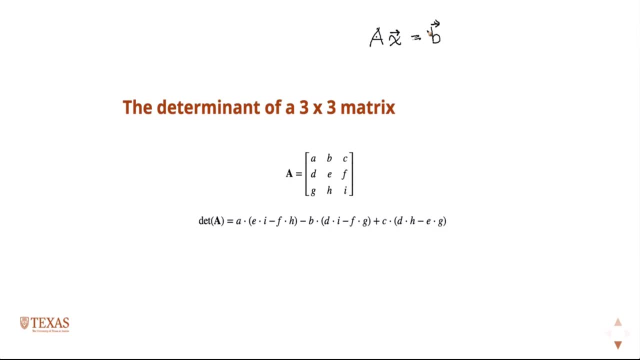 big matrix equations of this form, And so we're solving, we're looking for X in this way, and so the way you do this is you multiply, And it matters when you're doing matrices like so, if you're multiplying scalars, it 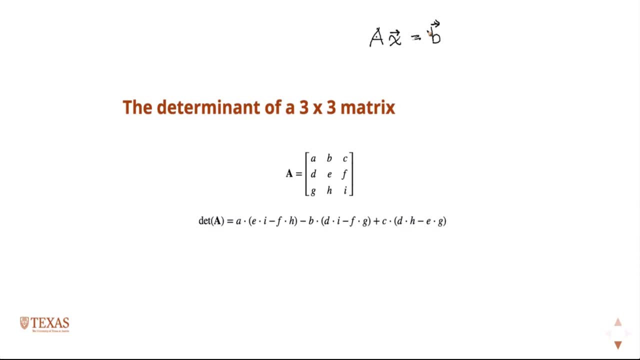 doesn't matter if you multiply on the left side or the right side of an equation, right, If I just multiply that equation by 2, I could say 2AX or I could say AX2, right, It doesn't matter. But with matrices it does matter on which side of the equation you multiply. 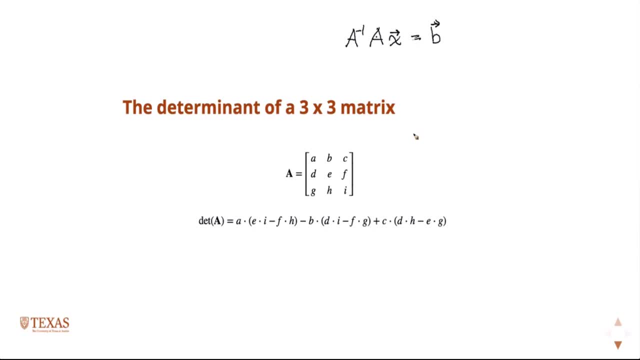 But if I multiply then both sides of the equation by A inverse right. any matrix times inverse is the identity matrix And any and the identity matrix times any vector is just the vector. So that's the solution to that equation. 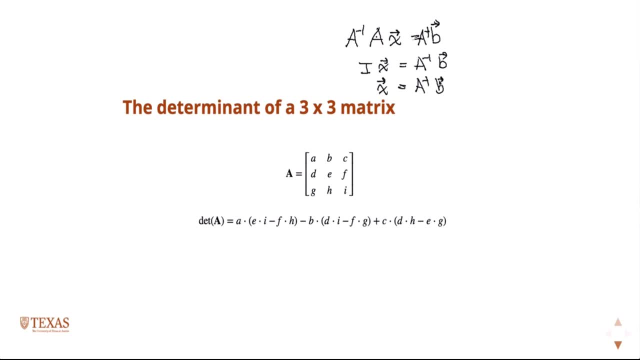 It's just. the thing is A inverse is not guaranteed to exist. Every you know, just because a matrix exists, it doesn't mean it's inverse world. And one way we can quickly determine so: if a matrix inverse does not exist, it's said: 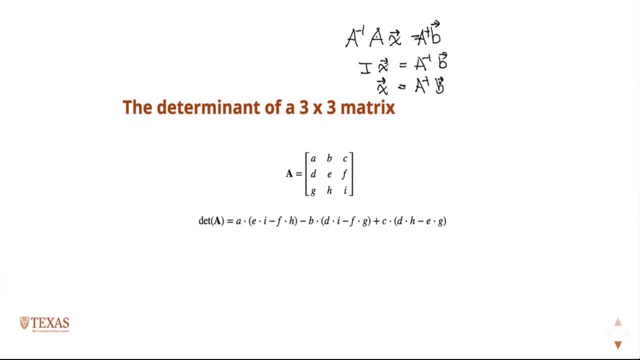 to be singular, And one way we can quickly determine if a matrix is going to be singular before we attempt to take the inverse, which is an expensive operation in a computer, is to compute the determinant. If the determinant is what, the matrix is singular. 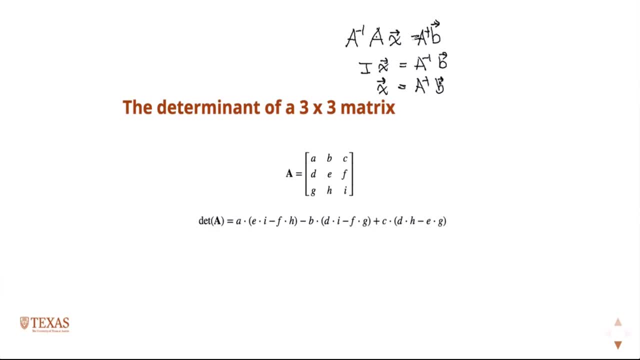 Anybody know If the determinant equals 0, so a matrix is singular if its determinant is 0. So in other words, if the determinant of a matrix is 0, it doesn't have an inverse And therefore this system of equations doesn't have a solution. 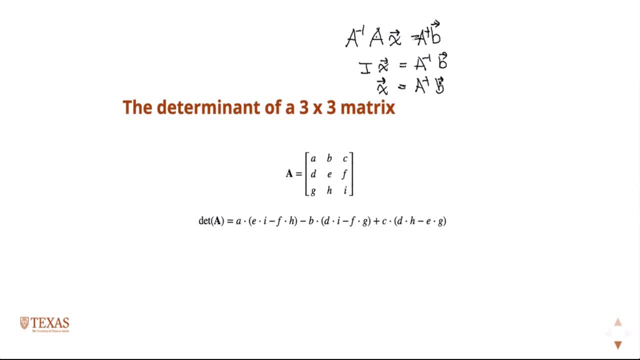 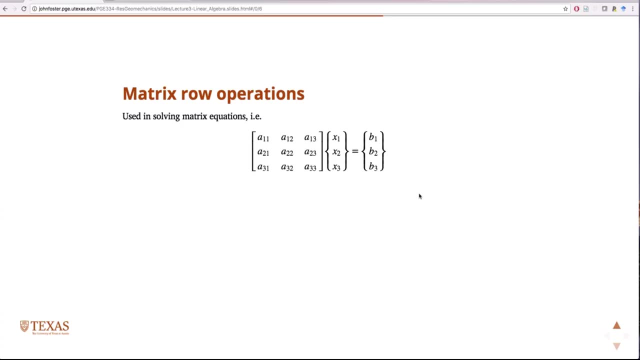 Okay, I think that's a good place to stop for today. So we're continuing our discussion of linear algebra Again because we're going to use this extensively in the class to solve for principal stresses, to do matrix-to-matrix multiplication, other things like that. 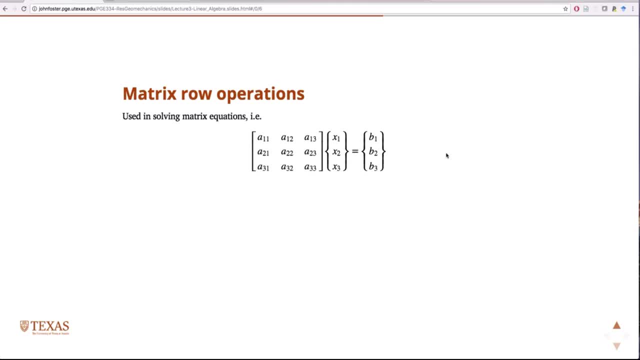 One of the most used, I guess, useful parts of linear algebra is in solving linear systems of equations. And so if we have a system of equations that we'd write in matrix form like this, we have a matrix. This would be A, This is a vector X, This is a vector B. We consider that we know all. 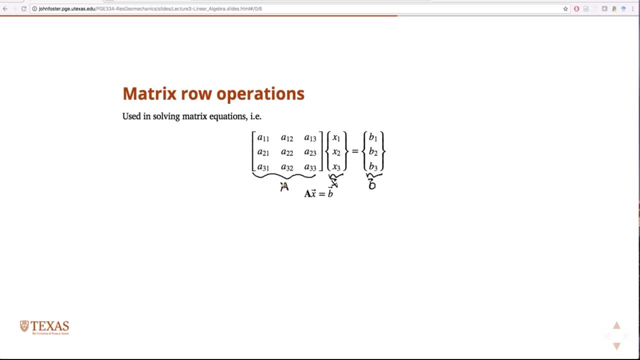 the components of A and we know all the components of B and we're seeking the solution to X, right? So this is no different than if we just wrote down a system of equations. So, in other words, if we did our matrix-to-matrix multiplication, we would have a solution. 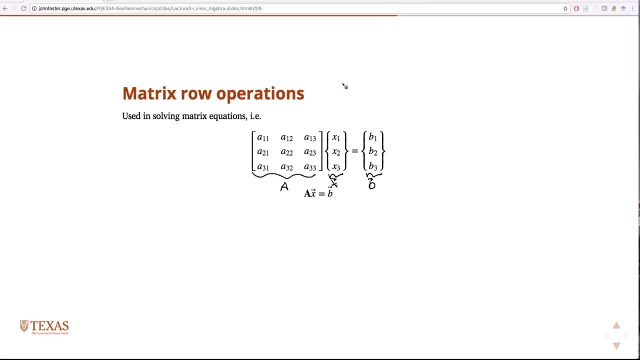 In other words, if we did our matrix vector multiplication on the left side- remember we talked about last time- so we'd have an equation: A11, X1 plus A12, X2 plus A13, X3 is equal to B1. 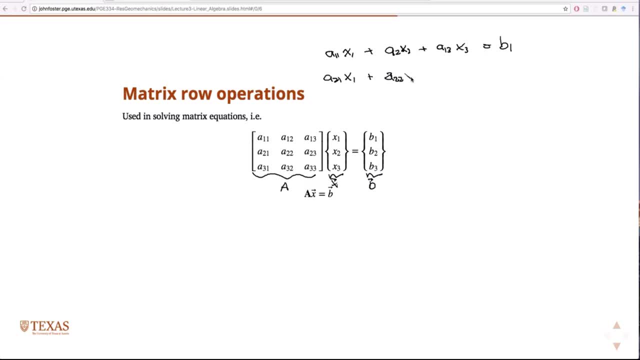 A21, X1, A22, X2.. A23, X3.. A23, X3 is equal to B2, and likewise for the last equation right. So when we solve matrices, solve systems of equations in this form, in the actual matrix. 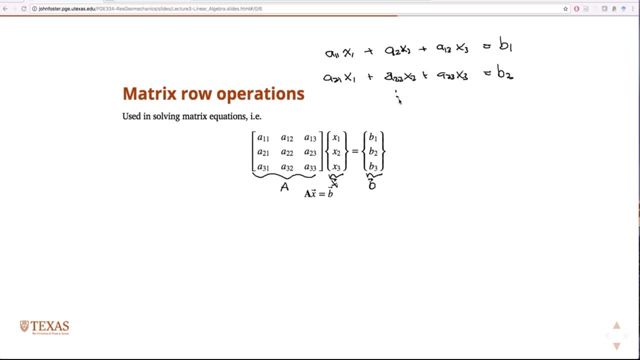 form. we can work through some things we call matrix row operations to do it for us and to solve these systems of equations, And they really just break down to kind of three rules. And the reason that it's nice to have these three simple rules is because we can implement. 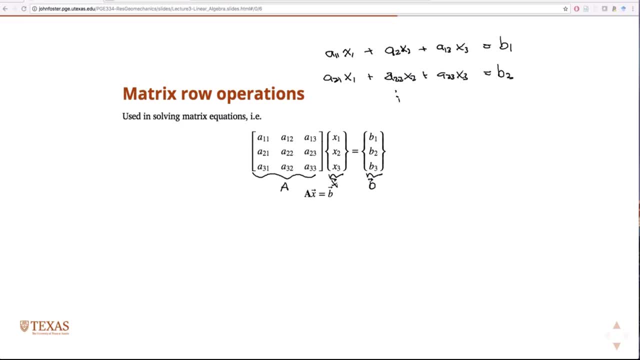 those three simple rules into a computer easily, And in fact whenever you have any direct solver that solves the linear system of equations in a computer, they just implement essentially these three rules Right. And so the first one is that swapping rows doesn't solve the linear system of equations. 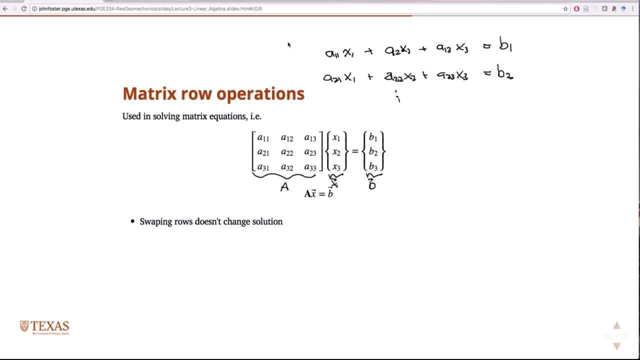 Right. And the second one is that swapping rows doesn't change the solution. And that should be obvious because- and that's part of the reason- I wrote out the first two equations, right, If this is just sort of a convenient way to write that and we were going to work out. 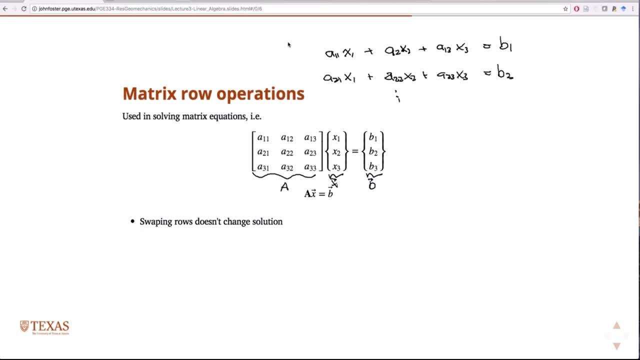 the solution to that linear system of equations by hand. of course it doesn't matter if I simply write the second equation on top of the first one, Which is essentially all I'm saying when I say that swapping rows of the matrix in solution vector don't matter. 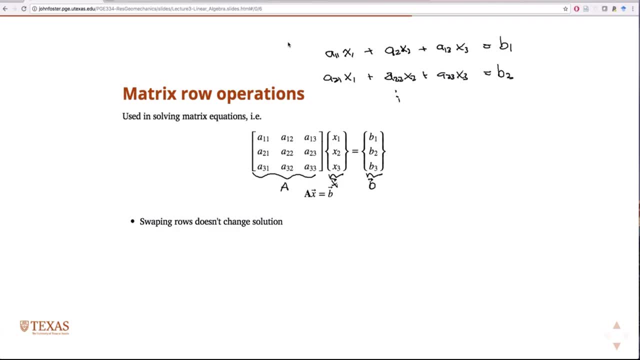 Right, Because it wouldn't matter if I just simply wrote one of those equations before the other, one Right, Adding rows together doesn't change the solution, So we often do this Like if you you know. these are things you've been doing since algebra two at least. 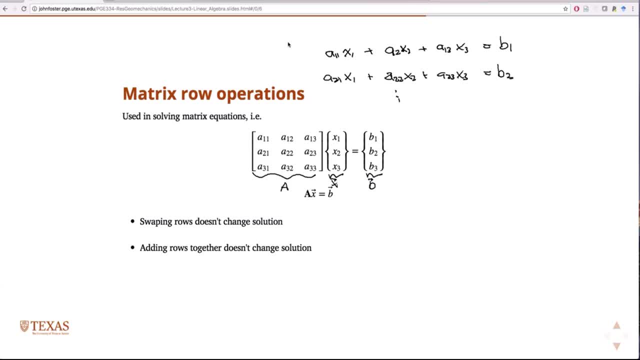 Right Or I guess, algebra You know since high school. Right, When you go to solve a system of equations, often you can just add the two equations together, because that will conveniently eliminate one of the terms. Right, And so we do this all the time. 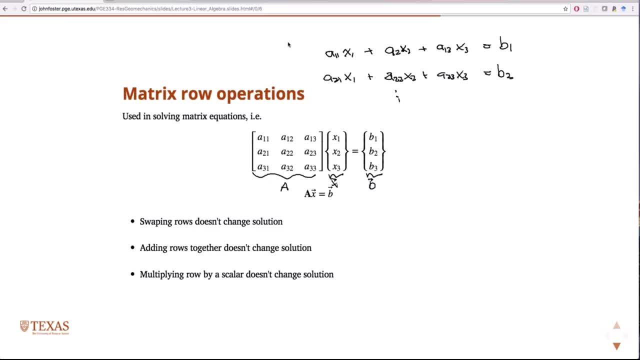 Multiplying a row by a scalar doesn't change the solution. Right? We all know this. If you have an equation and you multiply both sides of the equation by a number, it's still the same equation. It doesn't change the solution. 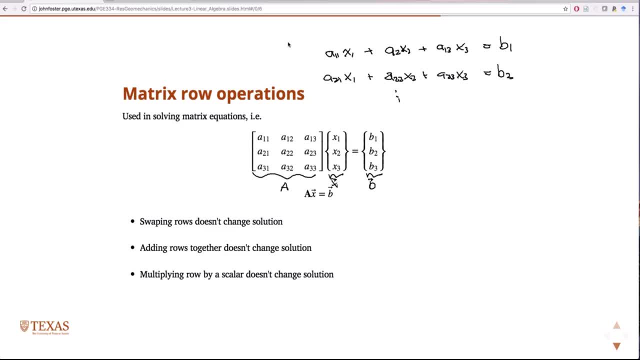 So we can solve linear systems of equations using some kind of linear system of equations, Using some combination of these three rules. And again, the reason it's nice to break it down is because this is the three rules we essentially implemented in a computer in a logical way. 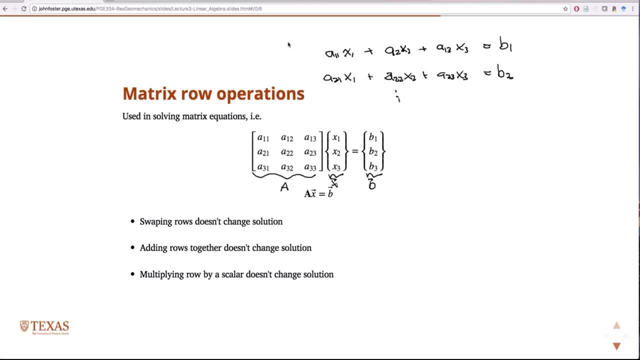 And we let the computer solve it for us. However, it's useful to do this at least once or twice by hand, because it gives us a convenient sort of set of tools for solving for something called eigenvectors, which we'll learn in about soon. 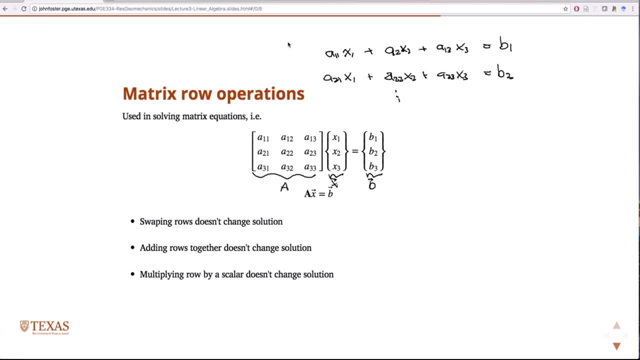 The next topic, actually. So let's look at an example. So this is our system of equations, written like this, And what we want to do is solve for X1, X2, and X3 using these three rules. Right? We call these row operations. 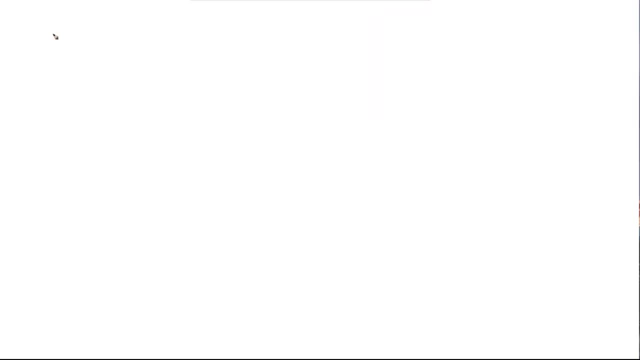 So I'm going to write the system of equations like this. So there's our A matrix And I'm just going to put a dashed line here And then I'm going to write the solution vector there. So 6 minus 6, 3.. 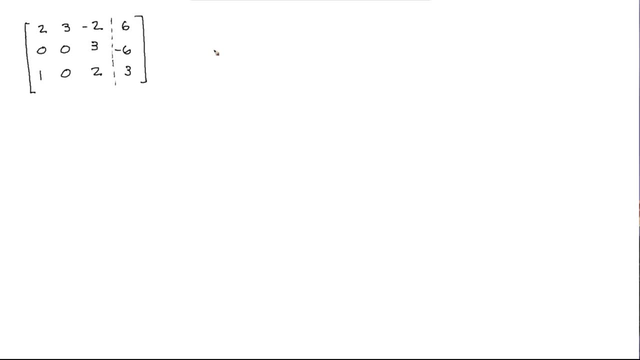 Right. So again, that's our system of equations, And I've just rewritten it like that. OK, Now what my goal is is to perform those row operations one by one, And it doesn't matter what order we do them. But I want to perform those row operations such that the left-hand side, the side on, 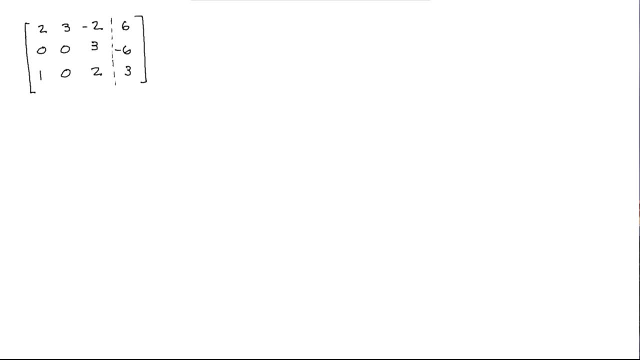 the left of that dashed line I wrote: Drew Becomes the identity matrix, So I just want a 1,, 1, 1 over there on the left-hand side. OK, So the first thing, and you know, as you practice this, you can, while it doesn't matter. 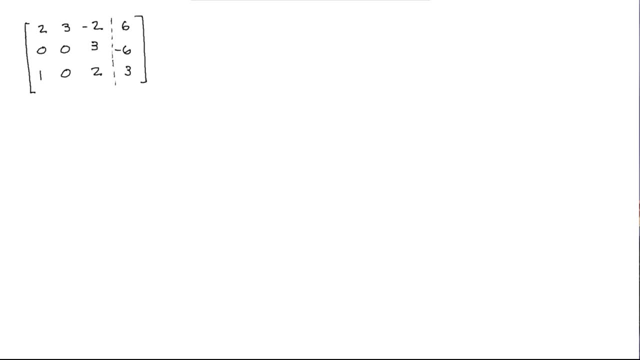 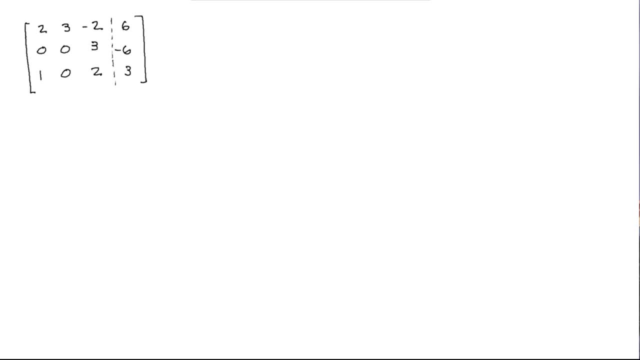 1 in the first row Right, And so this is going to be a little slow, I mean, especially for those of you that have seen this. but I just want to be very explicit And I'm not going to make you do this a thousand times in this class, but let's look at it. 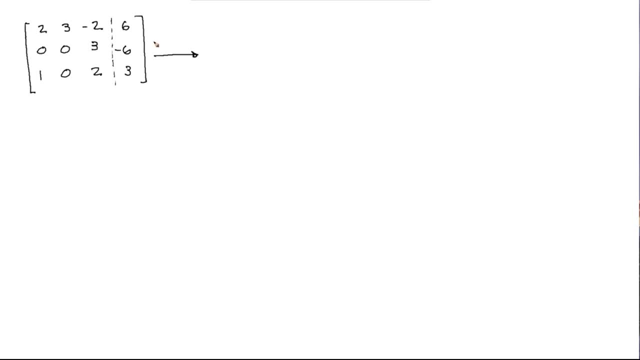 slowly, one time, Right. So what we're going to do is we're going to swap row 1 with row 3 and write out the results, So 1, 0, 2.. We'll leave the next row alone: 0, 0, 3, minus 6.. 2, 3, minus 2, 6.. 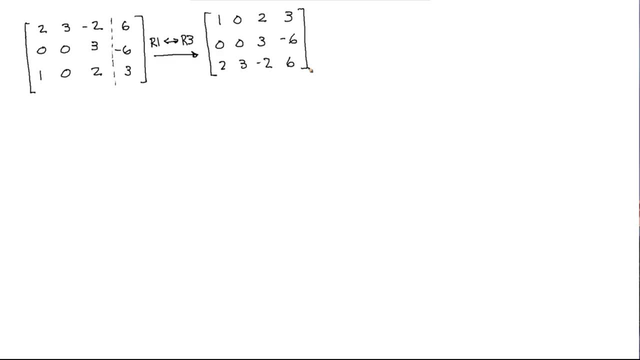 Okay, Now I'm going to multiply the second row by a constant right, By a number, And I'm going to choose that number carefully so that I can turn that 3, 0,, 0,, 3,. I'm going to turn that 3 into a 1.. 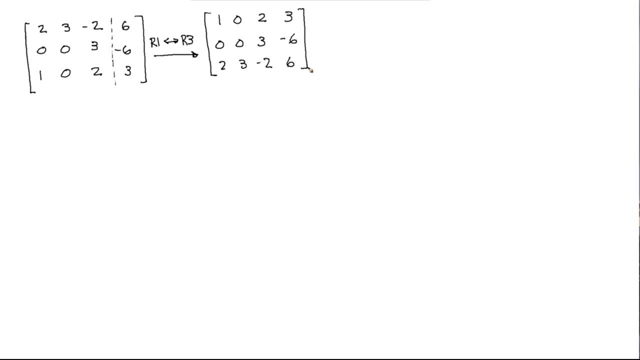 So what would I multiply by A third, right? So? So I'm going to multiply 1 third times, row 2, leaving everything else alone. And of course, as you get better at this, you can sort of do multiple operations at once. 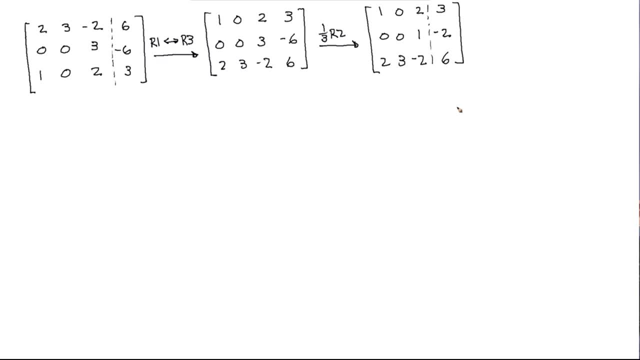 I'm not doing that. here Again, I'm going very slow, so you can see what I'm doing. So I just Again, I could have said I'd divide by 3, right, But dividing by 3 is the same as. 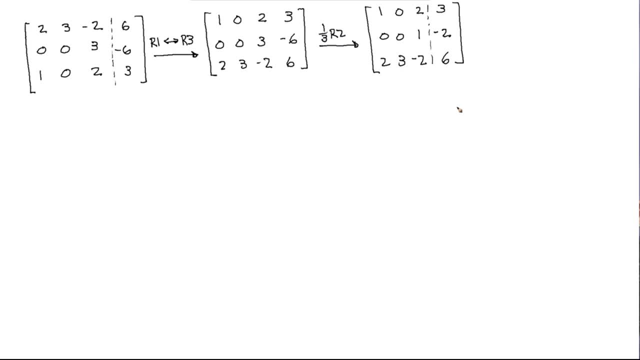 Our rule was multiply by a number, right? So we're going to multiply by a third. That keeps our rule simple, right? Okay Now, if I swap the second and third row, then I have a 1 where I need it to be right. 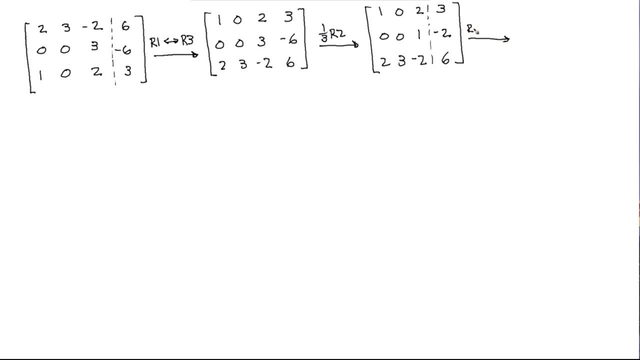 So Swap row 2 and 3.. Okay, Leaving everything else alone, All right, Okay, so now I will use kind of two rules and ones. What I want to do is I want to eliminate that 2 in the second row, right. 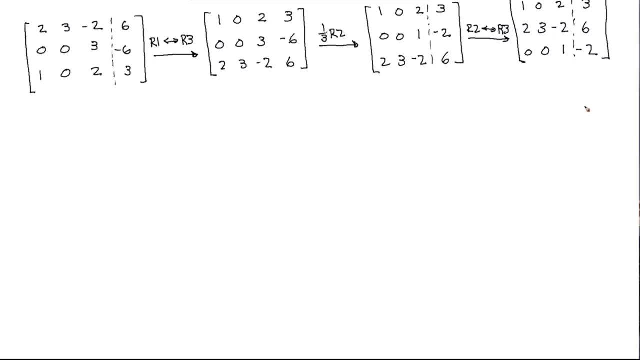 So what I'm going to do is I'm going to multiply the first row by minus 2 and then add it to the second row. Multiply the first row by minus 2, add it to the second row. So I'm going to say minus 2 times row 1 plus row 2.. 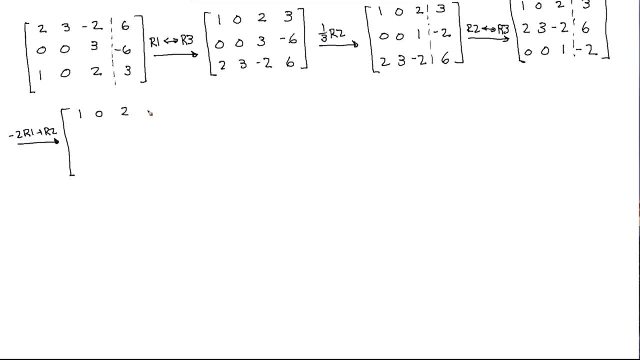 And that's going to give me. Everybody see what I did there. So minus 2 times 1 is minus 2, plus 2 is 0. Then I have minus 2 times 0, plus 3 is 3.. Minus 2 times 2 is minus 4, plus minus 2 is minus 6.. 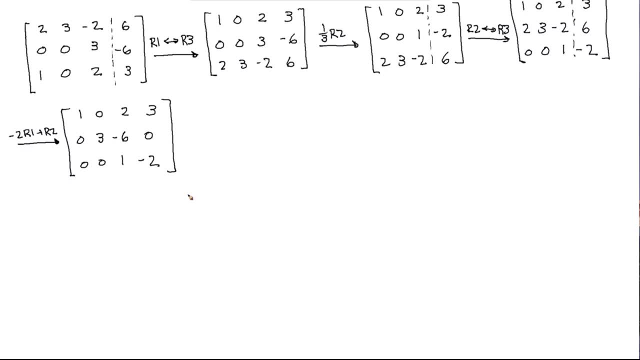 Minus 2 times 3 is minus 6, plus 6 is 0.. So that's how I went. I went from there to there. Okay, Now, if I divide this row by 3 or multiply by a third again, 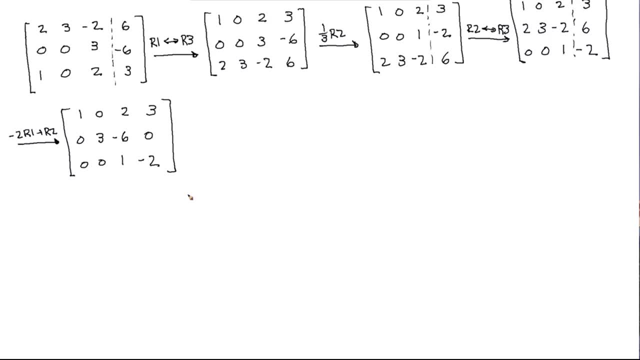 I'll have a 1 right there. So one-third row 2, 1, 0.. There, So this is almost always what I do When I do these. I try to make this left, you know, the thing left of the diagonal line that I stopped drawing. 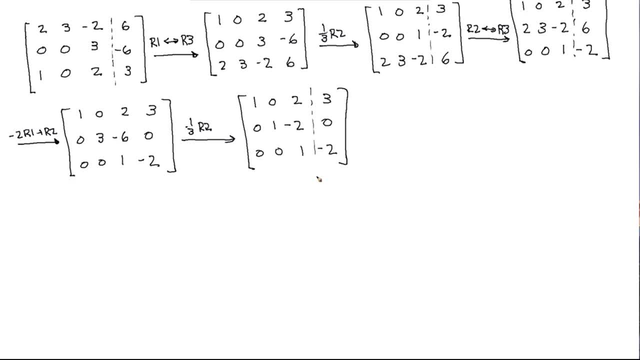 the horizontal, the vertical line that I stopped drawing there, everything to the left of this. I want to make this guy upper triangular right So that it has zeros down below One's on the diagonal And then it becomes real easy to eliminate above it. 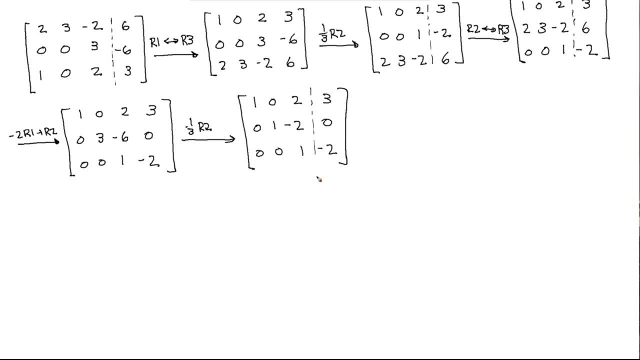 And, by the way, I mean we're working on a 3 by 3, but this works for a 1,000 by 1,000 matrix. This is exactly what a computer does to solve big matrices. So then, yeah, so then I can just eliminate above. 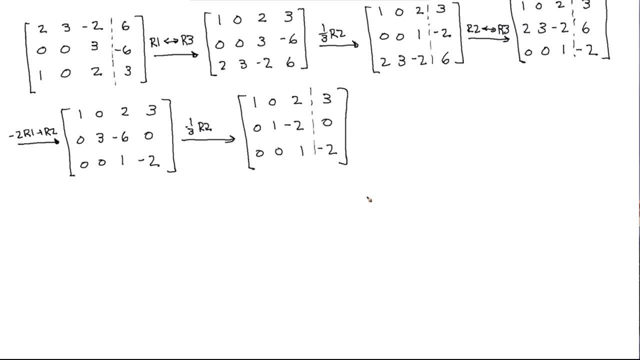 So 2 times row 3 plus row 2.. 2 times row 3 plus 2 times row 3 plus row 2.. Yeah, No, no, 2 times this row would give me a 2 there, and then I'm going to add it to that. 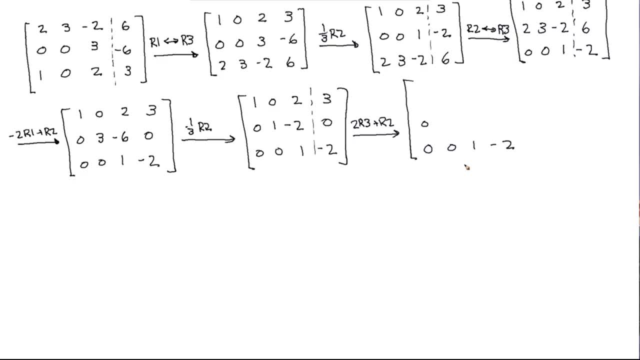 2 plus minus 2.. Yeah, Yeah, so, Yeah. so here I have 2 times: 2 is minus 4 plus 0 minus 4.. And then now on this last one, minus 2 times row 3 plus row 1.. 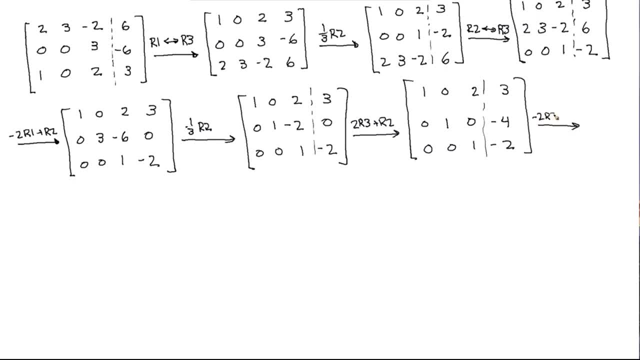 So now, minus 2 times row 3 plus row 1.. It gives me 1, 0, 0, 7, 0, 1, 0.. That's true, All right. So what's left? on the right-hand side? there is the solution. 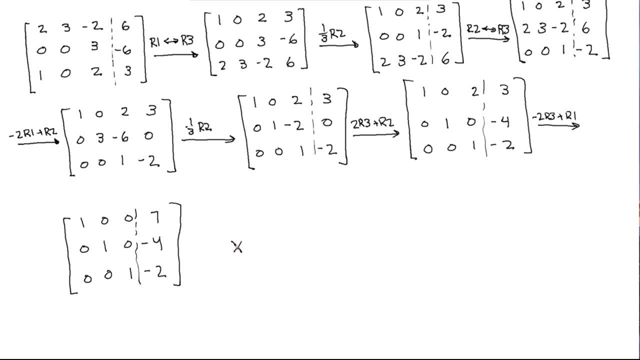 So my solution vector Is: X is equal to 7, minus 4, minus 2.. So in other words, X1 is equal to 7.. X2 is equal to minus 4.. X3 is equal to minus 2..